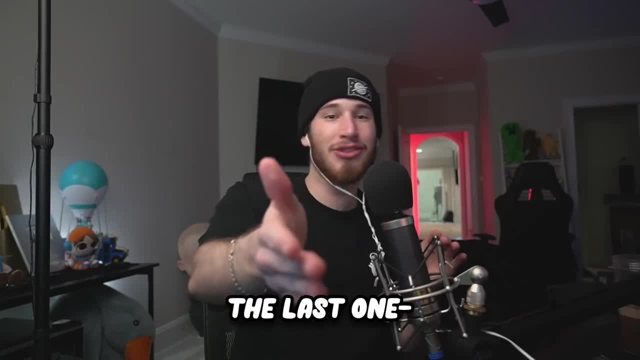 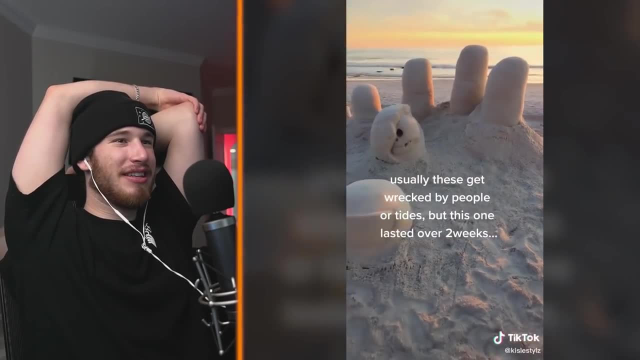 Today we're going to be checking out the craziest sandcastle creations. The last one is bigger than your house. What happens when a sandcastle is left for weeks? Bro, that's not left for weeks, Dude, it's died. Oh, that's funny. when you shower too long, How does someone even make that out of? 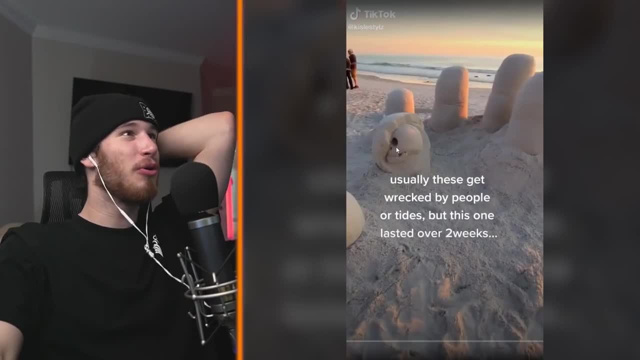 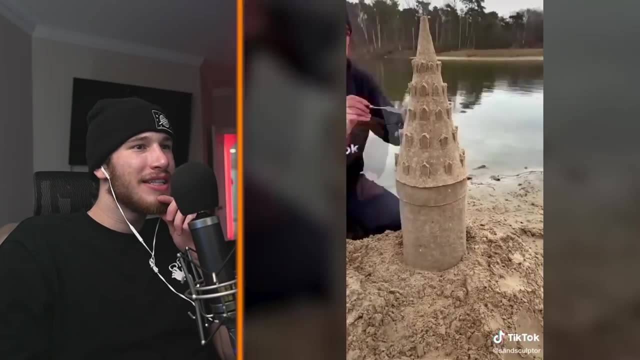 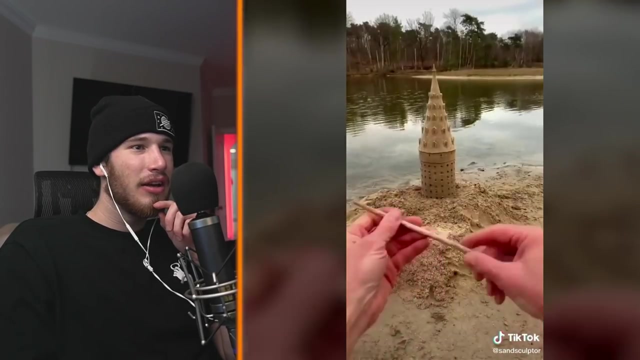 sand. What is that? Is that an egg with a skull? That's a skull with an egg. Sand Hogwarts, The whole wizard thing. You can't just say Hogwarts and make a cone. That's not Hogwarts. Is this a local lake? It looks like it. This guy sounds like a genius Magic tool stick. What You can't. 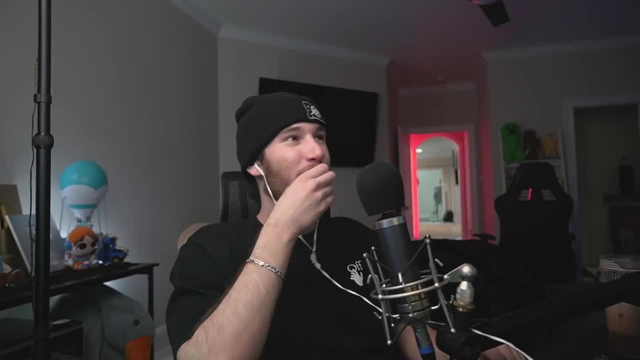 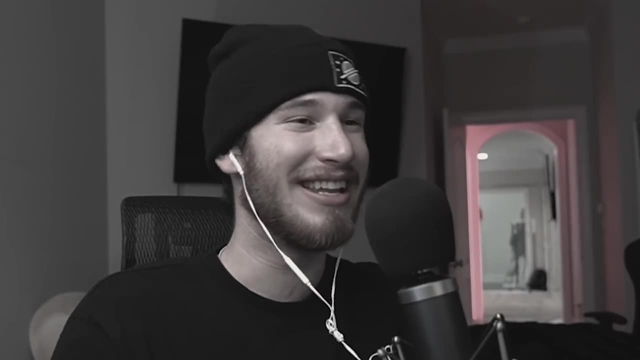 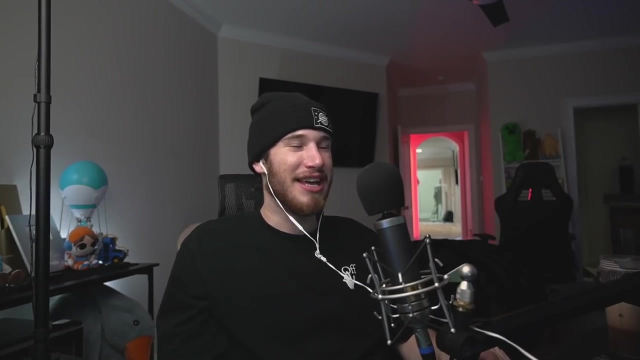 just wave a wand and have that happen. What kind of spell was that, Allie? What spell is that? He's a real wizard. You wouldn't understand. Okay, my bad, Millennium Falcon. How do you say it? Millennium Falcon? All right, what she said In sands. 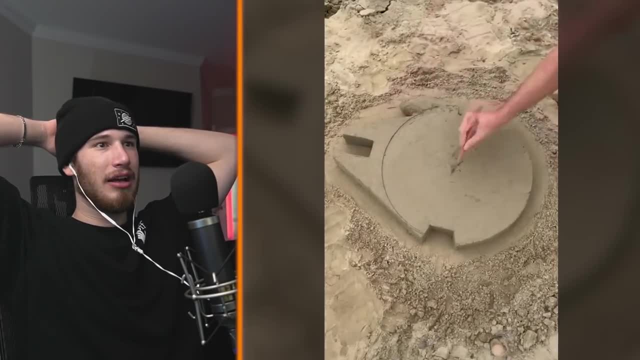 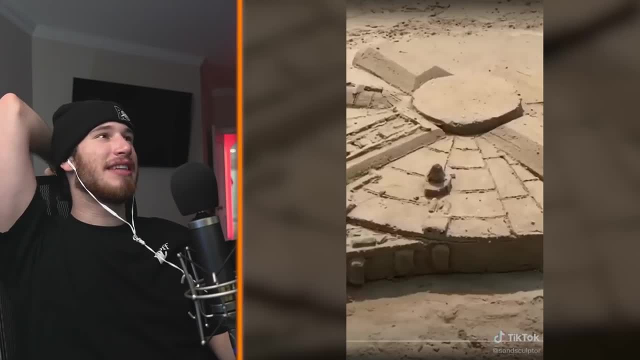 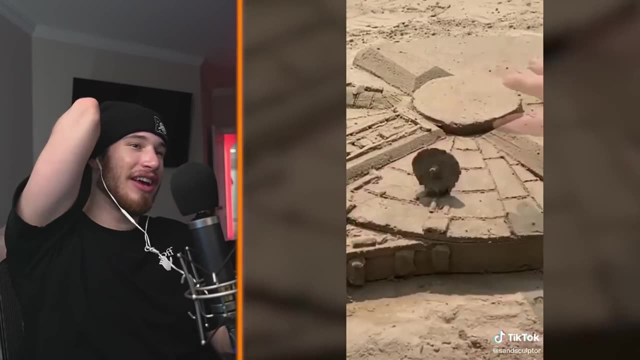 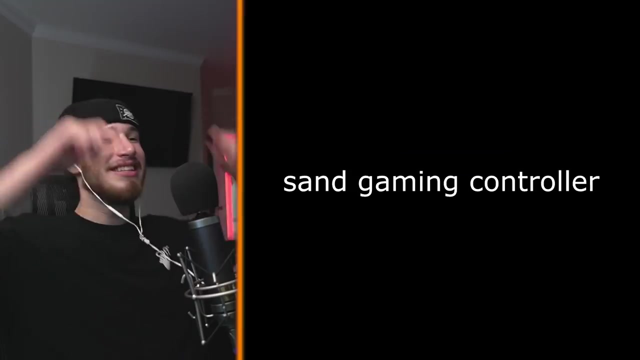 pancakes put on each other. Dude fly dog. Doesn't this guy get sad that after you make something like this it just disappears in a day? I mean, he got a video But it's gone. Wouldn't you want to keep this? Make it out of clay or something, Bro Sand gaming controller. 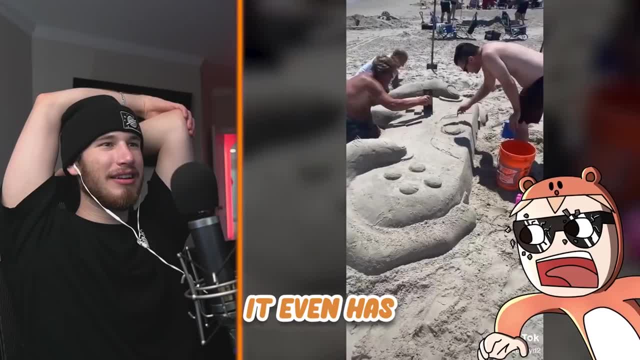 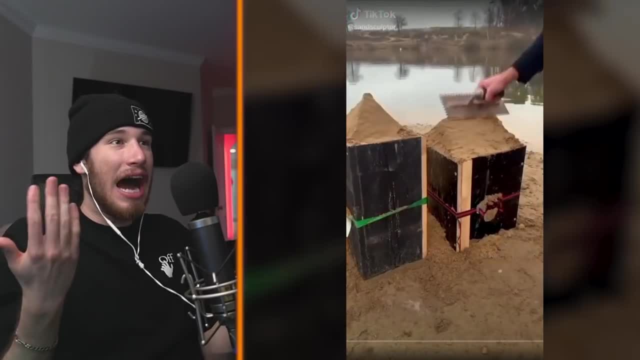 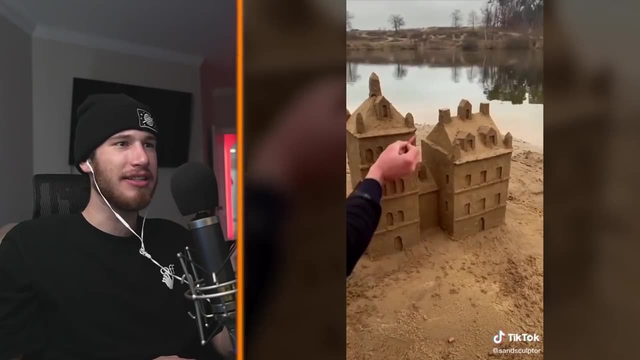 That's a big controller, Sand gaming. It even has hands. Gamers go outside once. Attack on Titan in sand. It's this guy. again It's the same guy. His whole TikTok is sand sculpture. That's his name: Sand sculpture. How's this attack on Titan? It's just a German house. 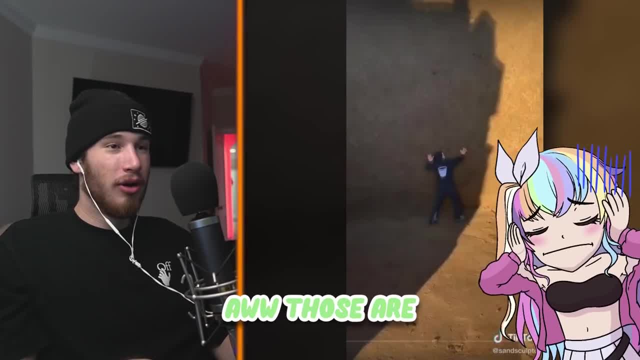 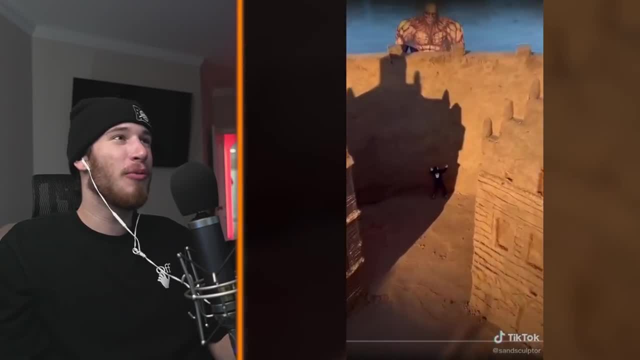 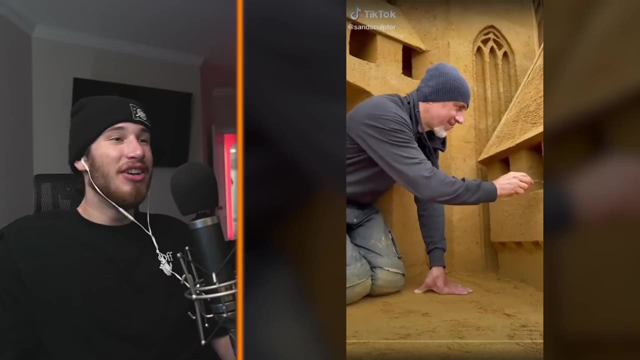 Oh, there's the wall. Yo, Oh, those are action figures. Why do you sound so disappointed? What's wrong with action figures? Allie, I wanted a sand Titan. Go watch Spider-Man. then Let me guess the same guy. No, this one is a massive sand castle. You're on to something. He lives there. 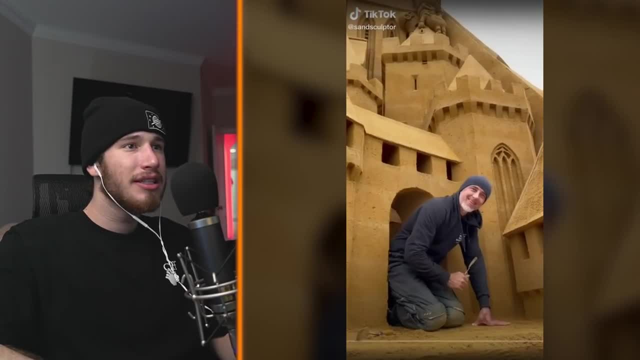 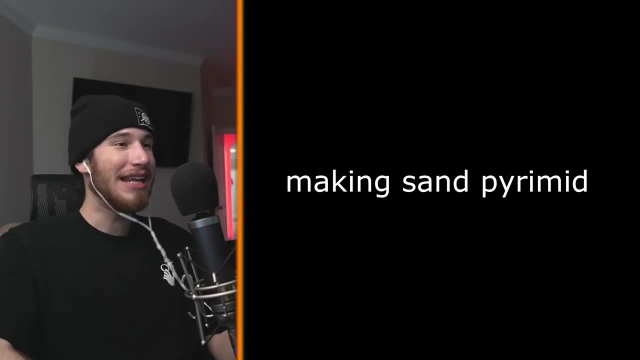 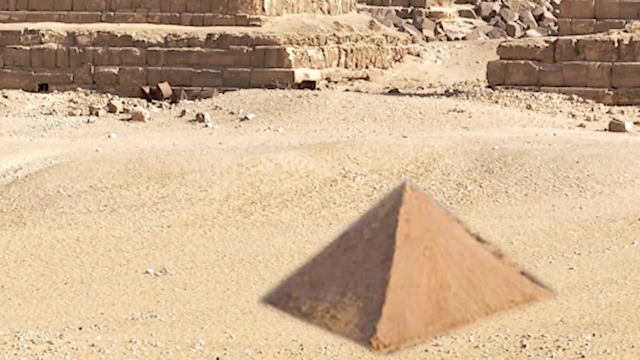 Dude, no wrench. This guy's so talented. Why do you find the sand for this? He stole everyone's sand. You go to your local beach and it's just empty. Making a sand pyramid, That seems pretty easy. I thought he was going to make a whole pyramid. You built it like right next to the 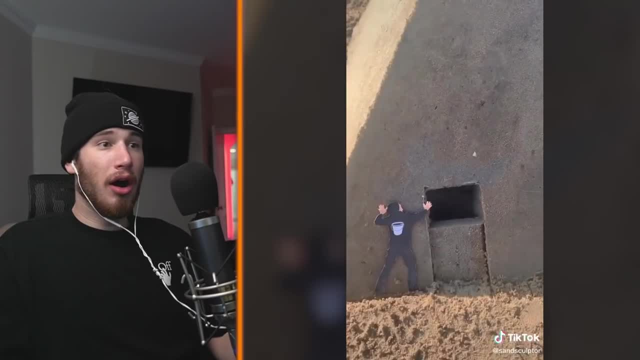 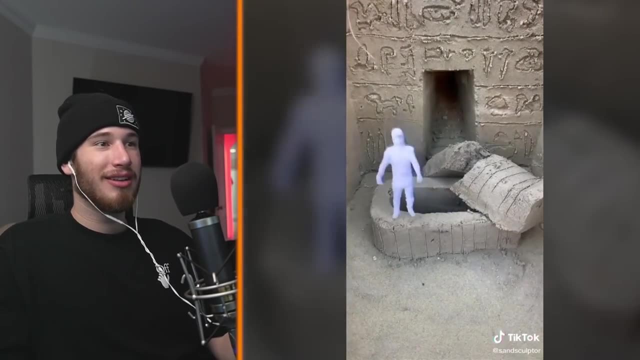 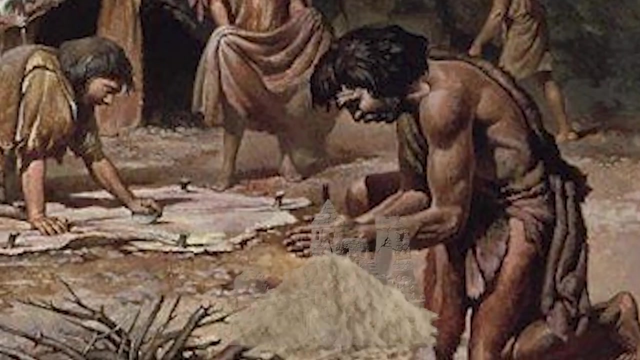 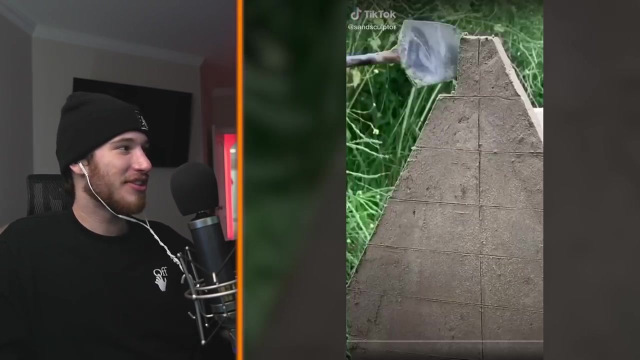 pyramids of Giza, Which was the real one. Oh, you can go in, Mommy. What the heck. So this is what people were doing before Minecraft existed. All right, that makes sense. Making a Dutch house. You're Dutch, right? Yes, This is your house, Is this? 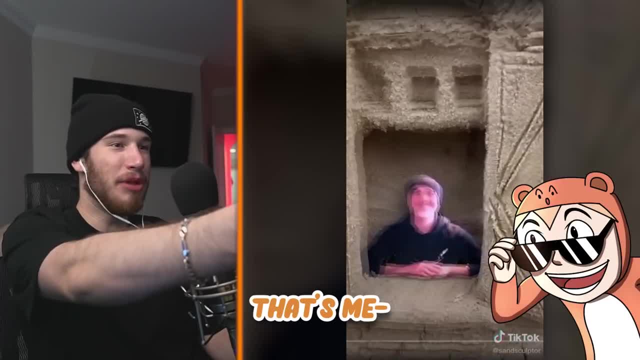 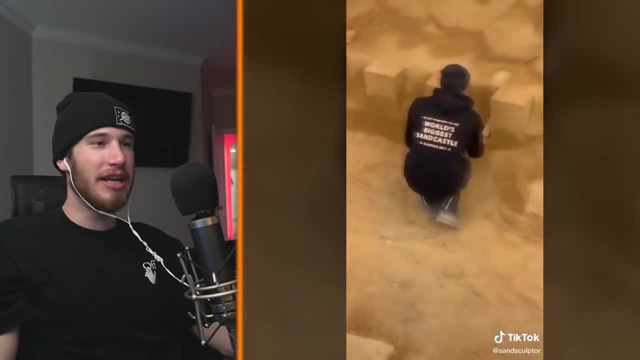 true? Is this exactly how your house looks, Blaza? Is that you? Is that Blaza face? reveal Massive castles. How massive, That's not That big. Oh, that's me. Oh, wait, wait, wait, wait, That's huge. 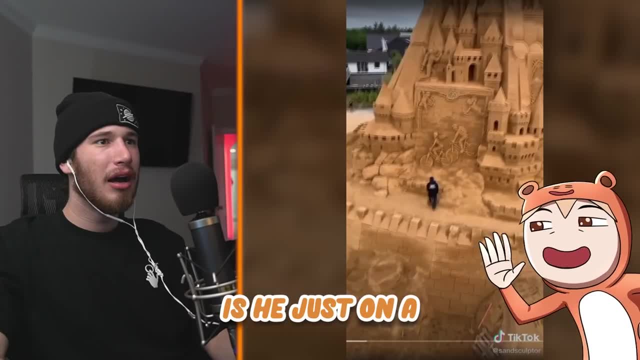 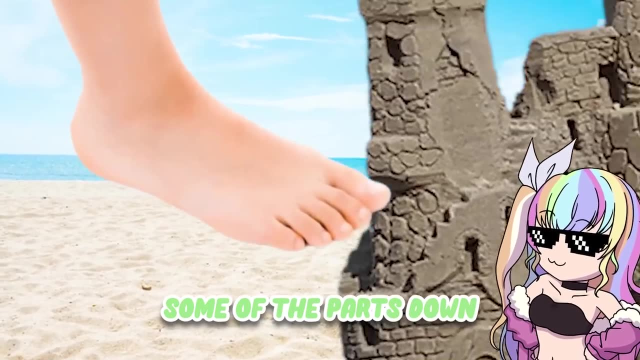 Ow, That's bigger than the houses in the back. Dude, is he just on a local beach? It's real. Imagine there's some kid going there every day, like kicking some of the parts down. When you mean kids Ally, you mean you right, You're the one going there and kicking some. 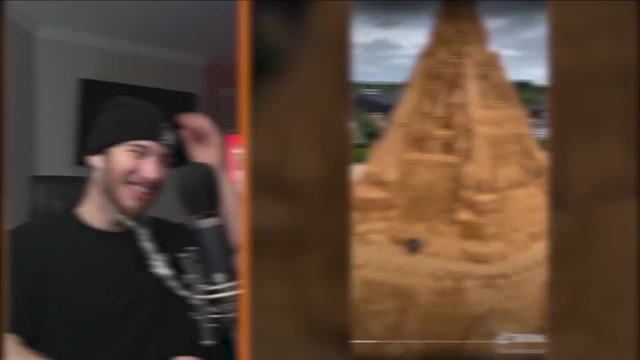 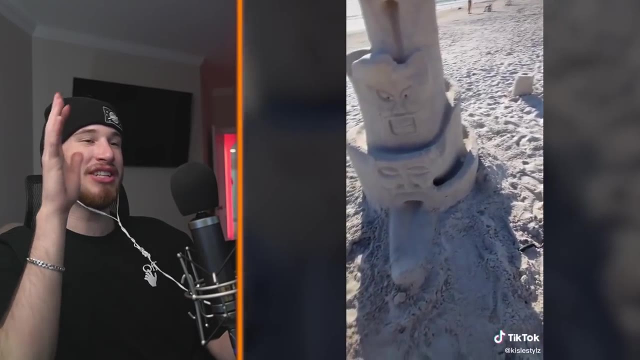 things down. Yeah, you bully Cool tiki structure. Hey, we play tiki Minecraft. Oh, and you can put a ball in it. Ball Ball, Mini golf. Imagine an entire mini golf thing, but it's out of sand. 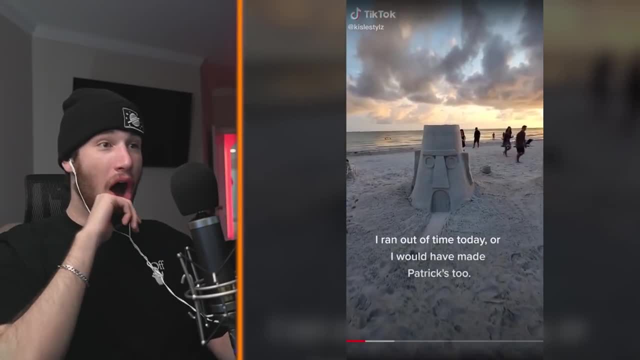 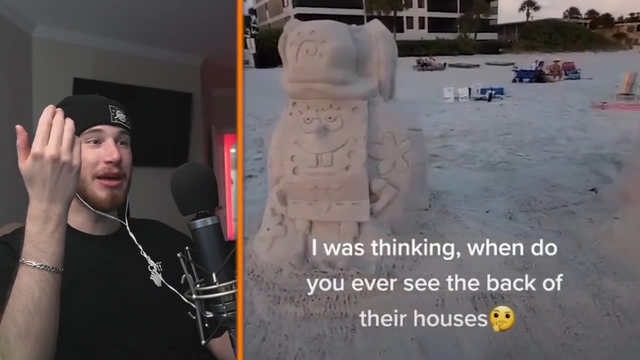 I don't think that was SpongeBob castle. No, SpongeBob, No, Oh Squidward, No way, No way. they didn't see Patrick's house. There's no way. Where's Patrick's house? I was thinking, Oh, when do we see the back of their house? Oh, 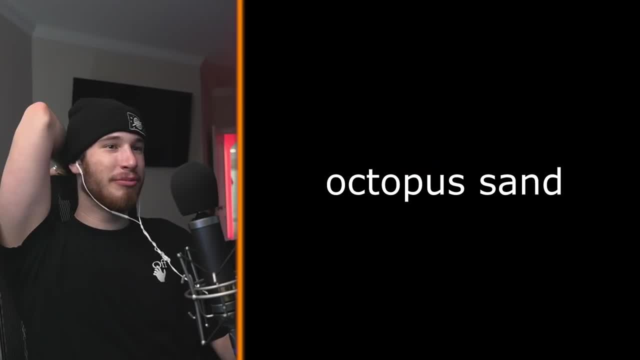 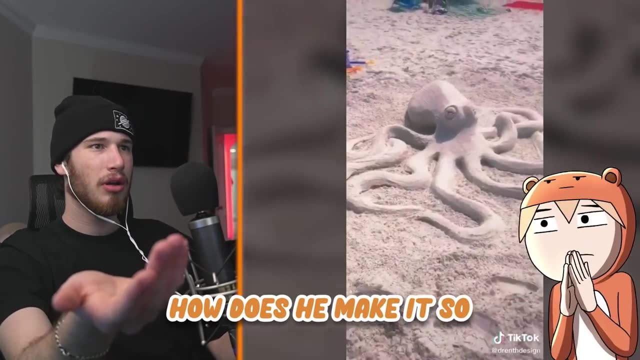 that's true. You never see the back of their houses. Octopus sand, That's a kid, That's a child. How is it so detailed, Like? how does just this guy know? How does he make it so smooth? Sand empire. 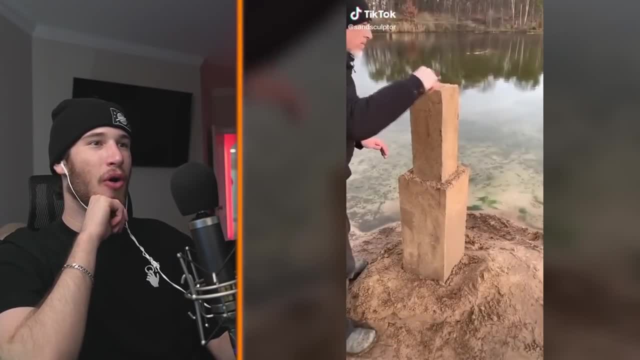 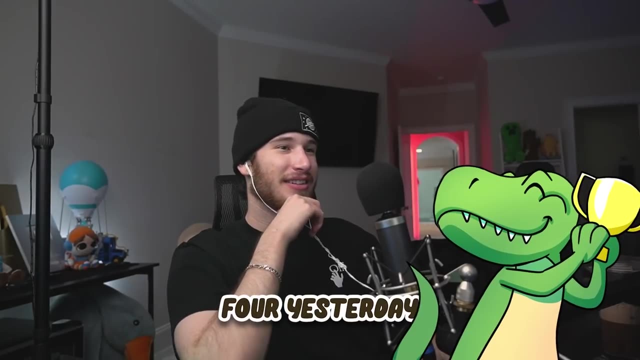 State building. Oh my God, This guy's bringing out the whole fortnight building kit. Anyone can do this. Dino, We know you did this yesterday, right? You're just being humble. I made it for yesterday Exactly. 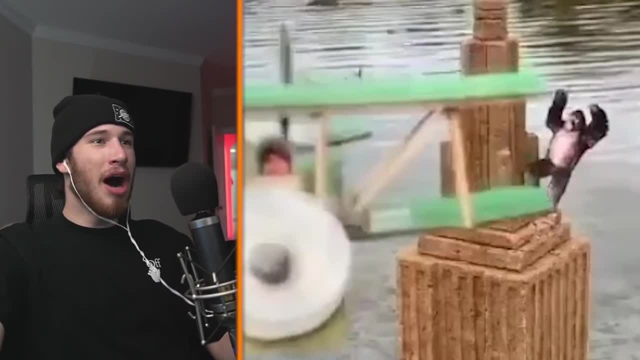 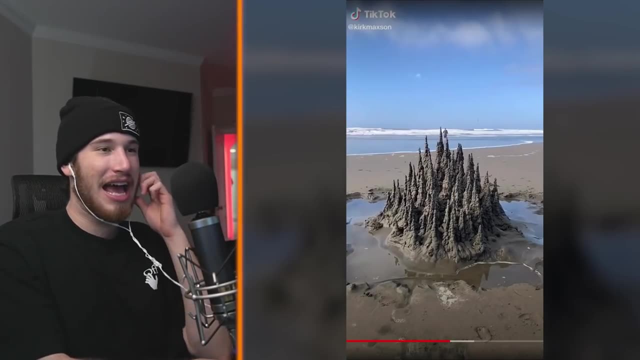 Exactly. Where does he get these planes? Monkey Destroying sandcastle. Allie, Oh my God. Allie cam, Allie cam, Oh my God. She's coming for the sea. Death of the sea, Oh no. 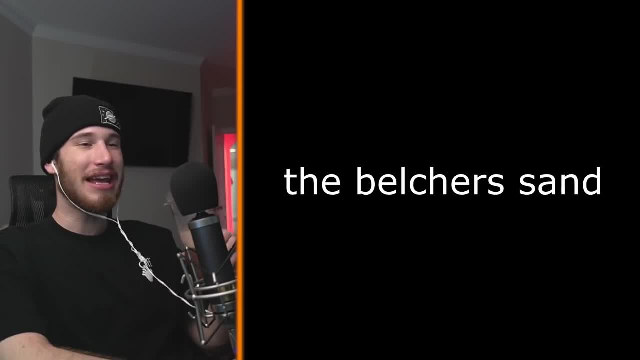 Oh, Oh, my God, The Belter sands. Wait, is that Bob's Burgers? What's that show Bob's Burgers, Bob's Burgers. It is Bob's Burgers. right, Yeah, that's Bob's Burgers. 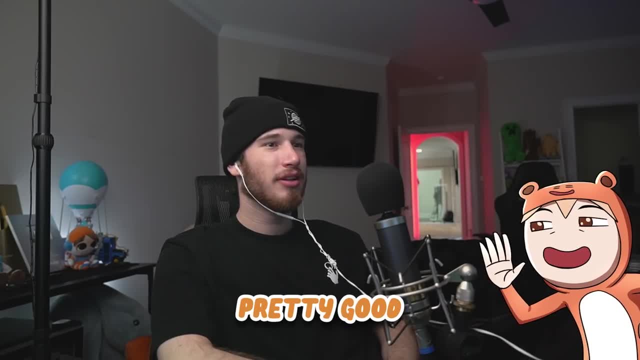 I watched like one episode of that. Is it good? What do you mean, Dude? it's pretty good. It's pretty good Burgers, and then it's called Bob. You never watched it, did you? I did like four episodes. 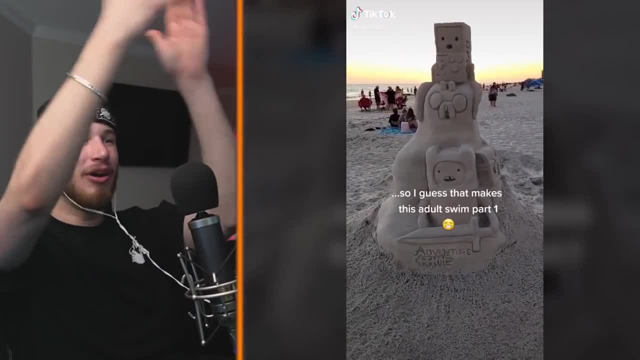 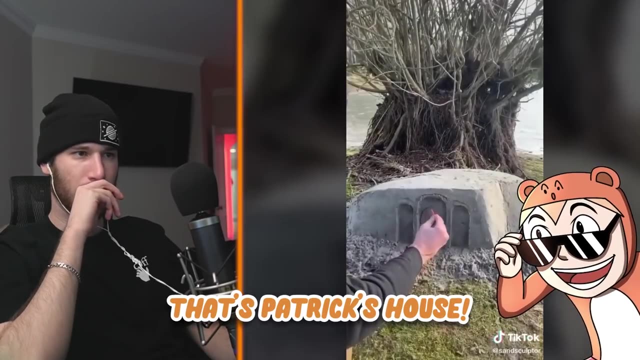 Adventure time. Yes, Yo, Bimo Dude, Jake is melting. Nah dude, his body's just morphed like that Lord of the Rings house. That's Patrick Patrick's house. I'm a big fan of Lord of the Rings. 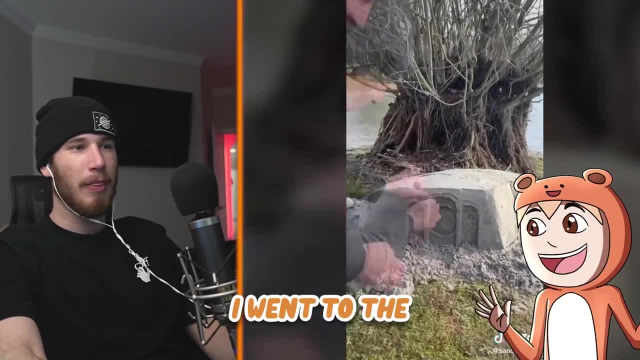 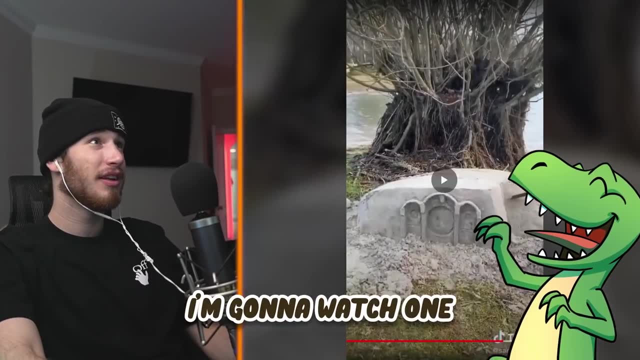 I just wish the movies weren't like 13 years long. I went to the movie theater for The Hobbit like four hours. I fell asleep. I was like I'm going to watch one before I go to bed And it was like five hours. 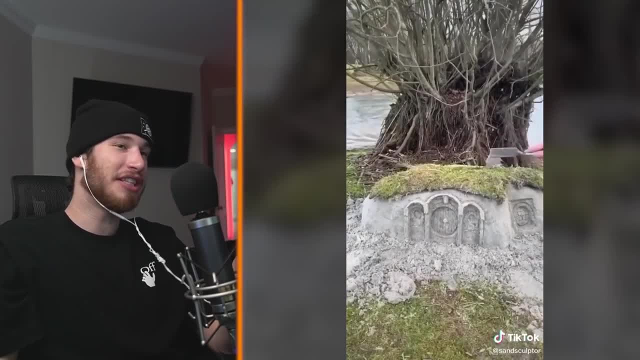 Five hours. Yeah, that's so good, Dude. Bilbo could actually live in there. That's what's crazy about that, Whoa, He made it inside. Oh my God, there's an inside. Here's a little candle. 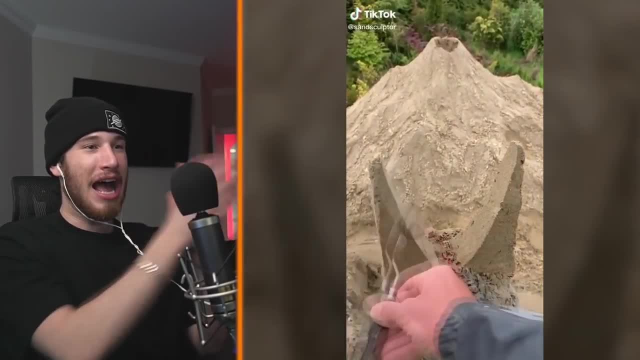 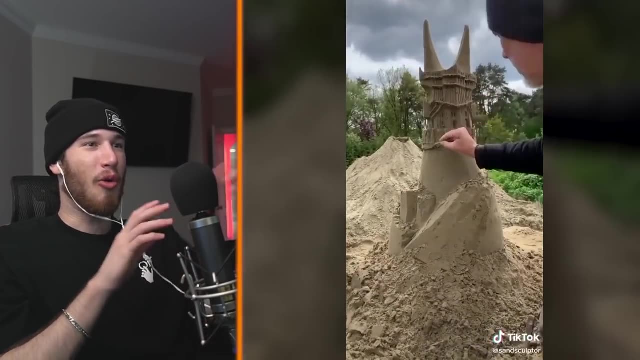 Tower of Mordor, sand Yo, the eye of eye, The ender eye, The eye of Salamanca. No, Salam Sala, Sauron, Sauron, Salamander Girl, don't look at it. 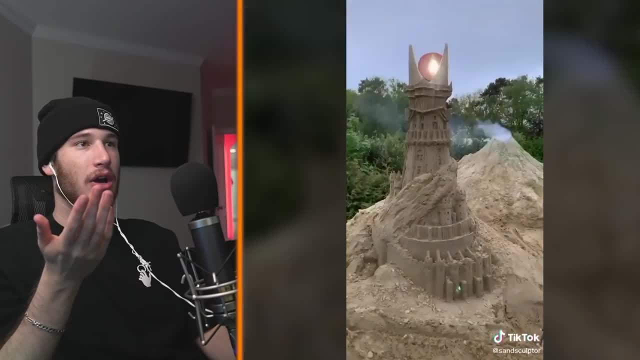 Don't look at it. Don't make eye contact. Don't do it. Wait, how is he going to do the eye? Whoa, That was real. Don't look though. Don't look, You'll get possessed Sand clock. 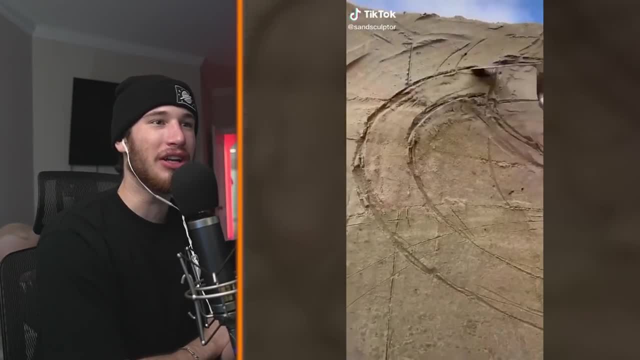 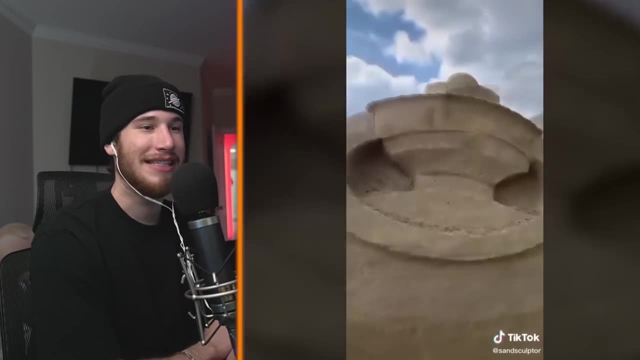 Sand clock. A full on clock. He's building the whole big den. Oh, They should hire this man to fix it. Let's go to the store. We need a clock to know the time. Sand guy, I got you Right outside my house. 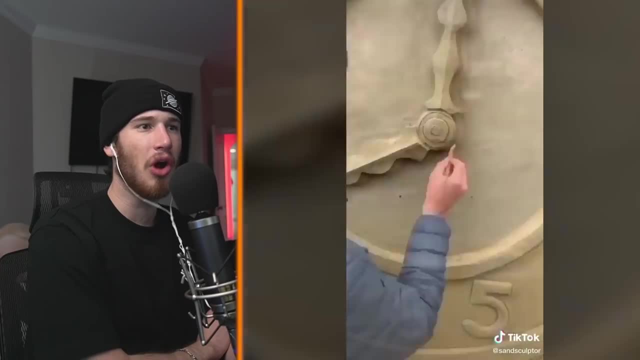 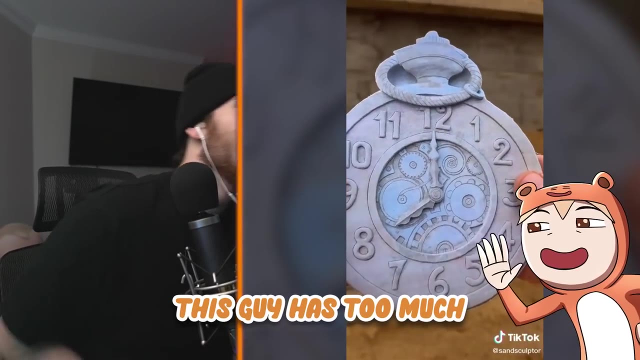 Oh Wow, That looks detailed. That looks so good. It even has a mechanism And it actually works. This guy has too much time on his hands. You guys better smash that subscribe button with that joke. If you don't, I swear to God. 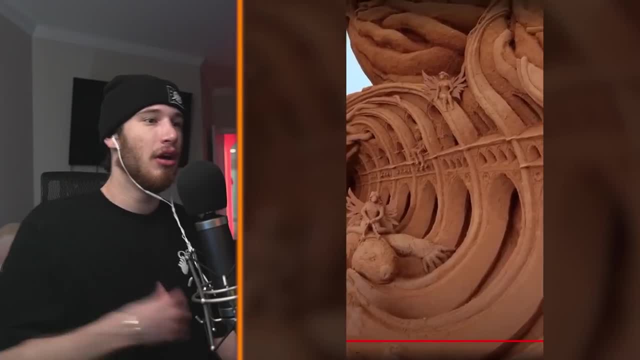 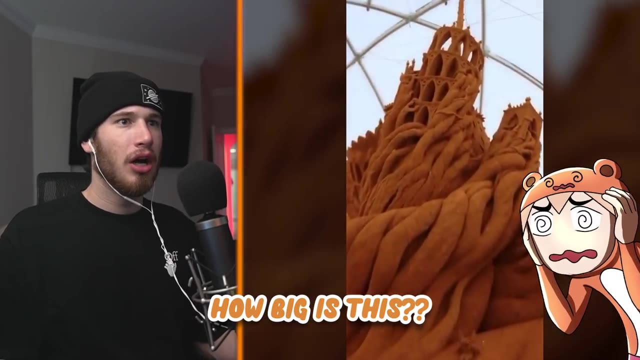 Insane castle- More insane than we've already seen- The freaking Mona Lisa, The whole forest. What, How big is this? It's got a dome. Is that a sand fairy? Let's wait, Let's do some size comparisons.